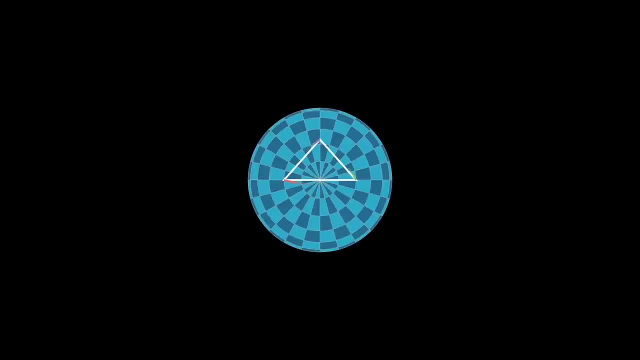 we find the angles of triangles adding up to more than 180 degrees. This is kind of understood better if you consider the curvature of the earth or a sphere, As weird as that might be. there's an even weirder number of angles that can be drawn on a sphere, And that's because the 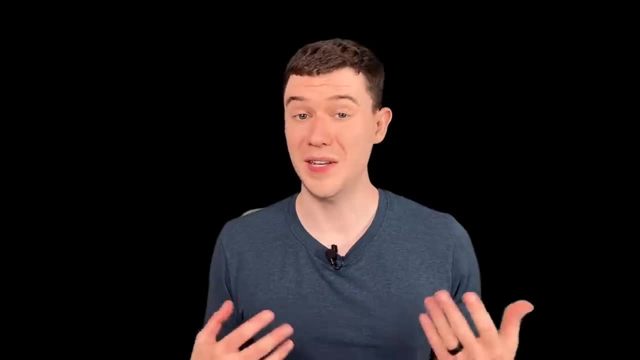 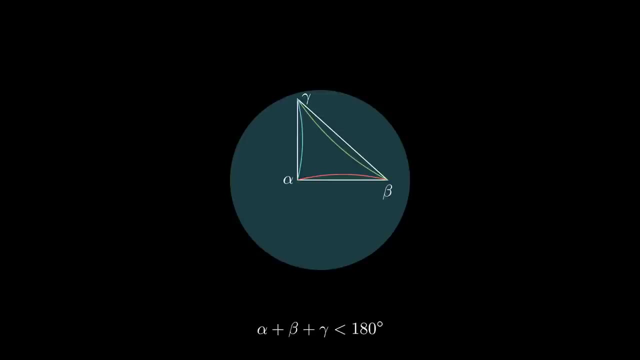 angles of triangles are drawn on Euclidean geometry, known as hyperbolic geometry. In this geometry- you guessed it- the angles of a triangle add up to less than 180 degrees. Here, imagine triangles being drawn on hyperbolic surfaces like Pringles chips. Did you ever notice? there's no Roman. 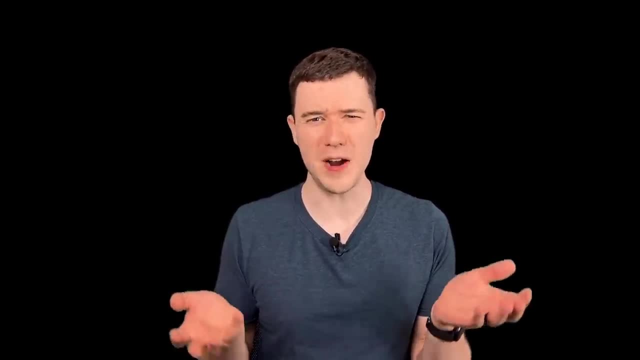 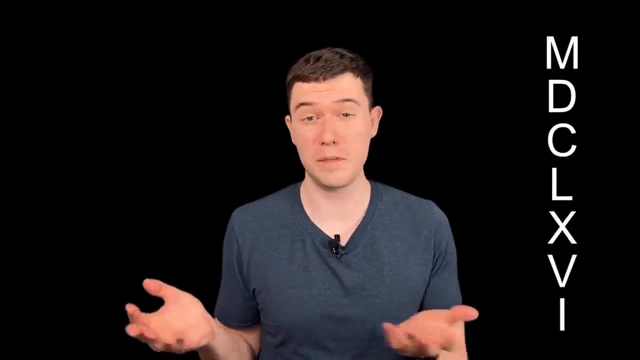 numeral for zero. That's right. if you try to write the Roman numerals, you'll see that there's no way to indicate an absence of something. This highlights an important part of mathematics history: that zero wasn't always the right number. If you try to write the Roman numerals, you'll see. 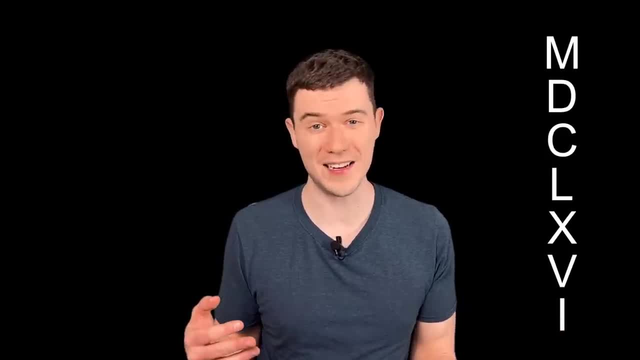 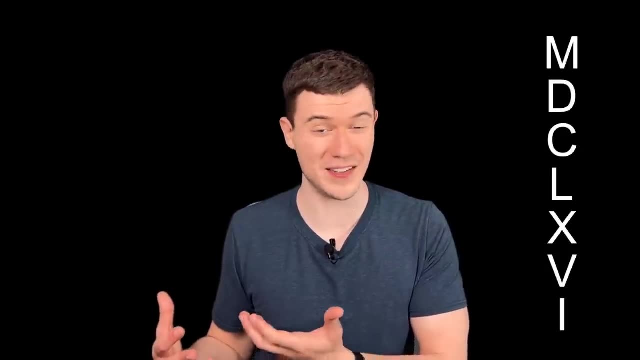 that there's an absolute opposite of what you'd expect. The Roman numeral system was an additive system Using I's, V's, L's and so on. it lacked a lot of the nice mathematical properties that we take for granted today. The Mobius strip is a fascinating geometric object. Take a long rectangular. 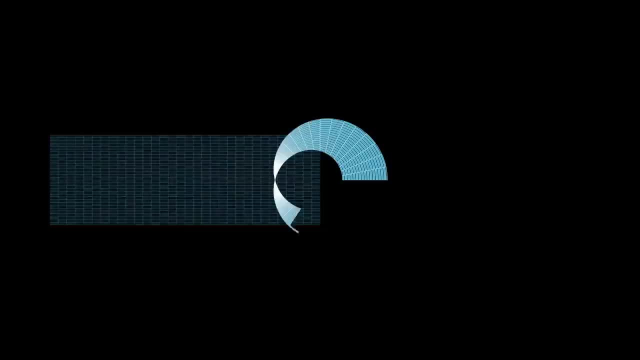 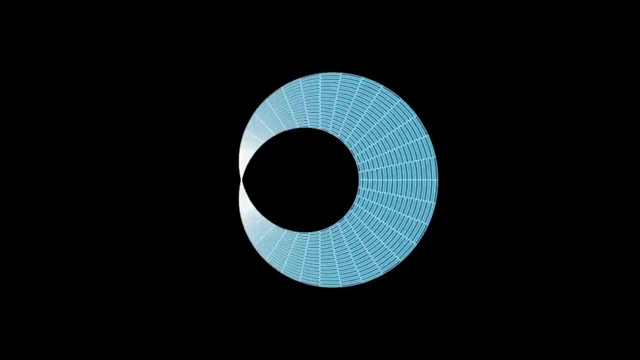 piece of paper, give it a twist and attach both ends. You've just created a one-sided object. It's essentially just a continuous loop with a twist, but it has a ton of cool properties and is pretty cool and it's a great introduction to topology. 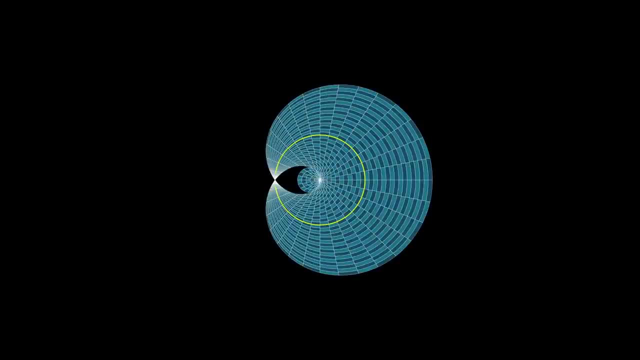 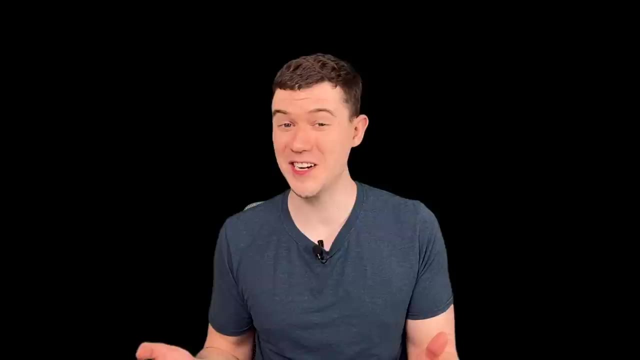 If you were to draw a line along the center of the strip, you'd eventually return to your starting point, even though there's in fact only one side. It's a pretty captivating geometrical object and really kind of defies our understanding of how surfaces and geometry works. 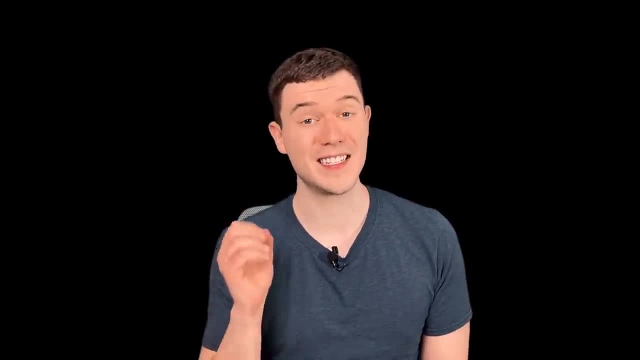 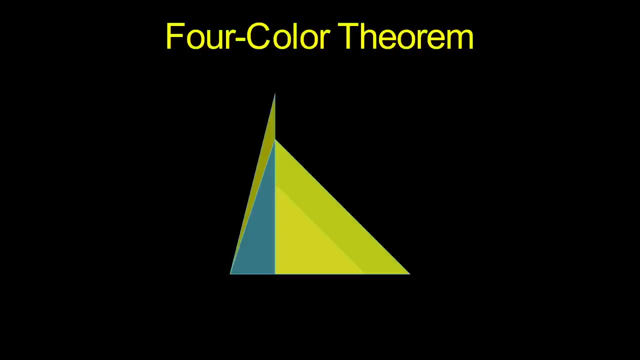 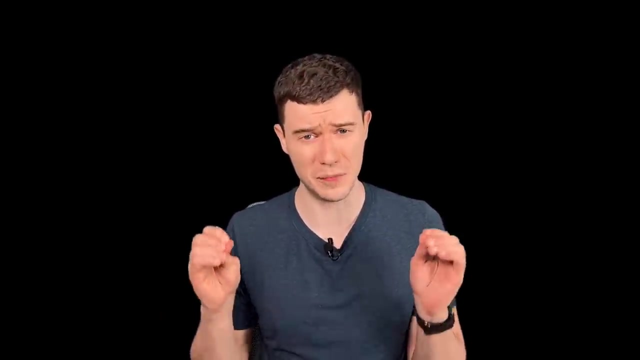 The four color theorem is a famous problem in math. that states any map can be colored using only four colors. Did I mention it's in such a way that no two adjacent regions have the same color? Now, it was proven in 1976, but it took a ton of time and computational power. 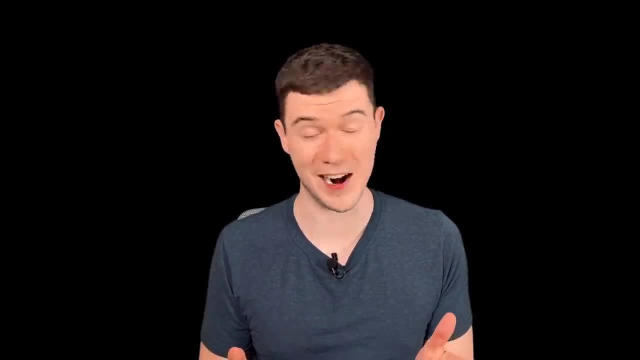 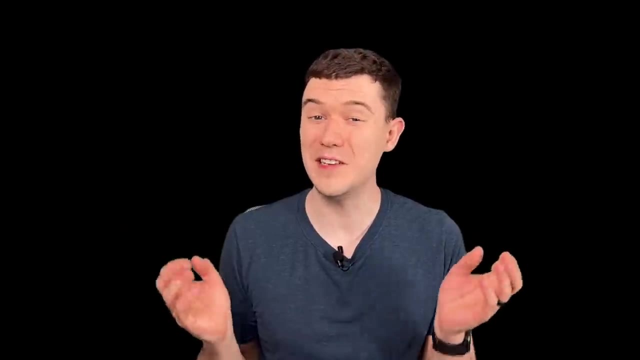 And when I say computational I mean computer power, and that was kind of a big deal back in the day, Given that it was met with a lot of skepticism and criticism, but now it's universally accepted and has significantly impacted things like graph theory and combinatorics. 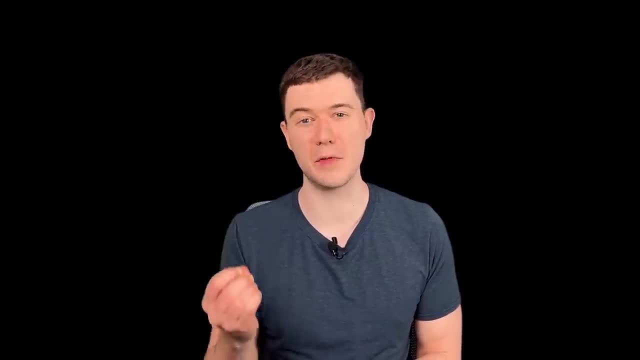 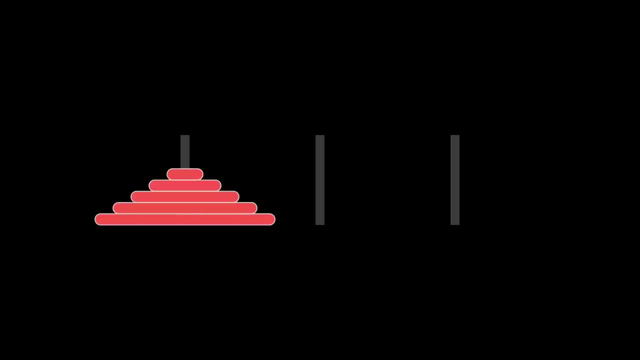 The Towers of Hanoi is a famous puzzle made up of rods and disks. The puzzle starts with the disks in a stack in ascending order, and the objective is to move the entire stack to another rod. Only one disk can be moved at a time. 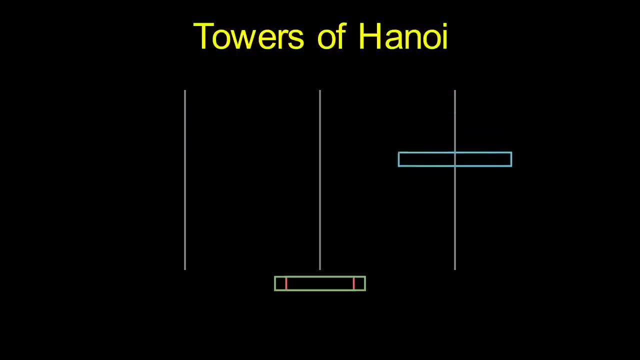 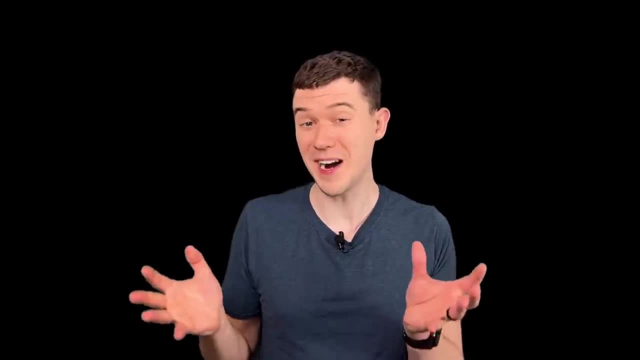 Each move consists of taking the top disk from one of the stacks and placing it on another rod. No disk can be placed on top of a smaller disk. Now, the beauty behind this is in its simplicity, yet its complexity. There's a nice mathematical formula. 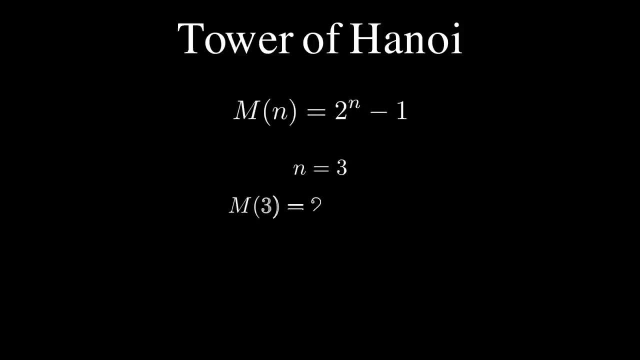 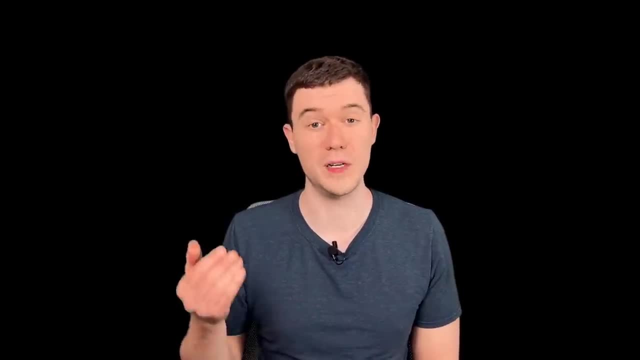 for the minimum number of moves to complete the game. It's two to the n minus one, where n is the number of disks. So the minimum number of moves to win with three disks would be two to the third minus one or seven moves. 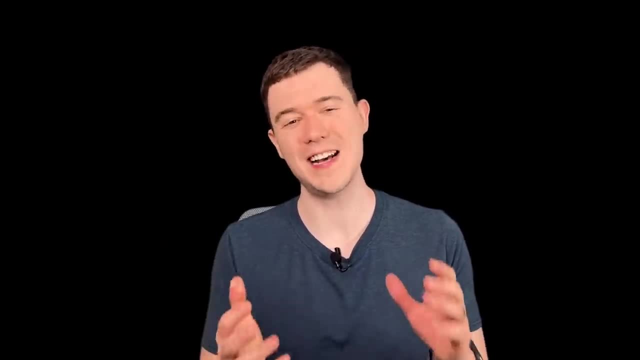 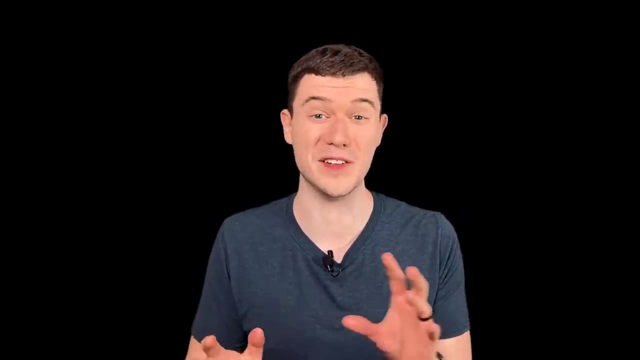 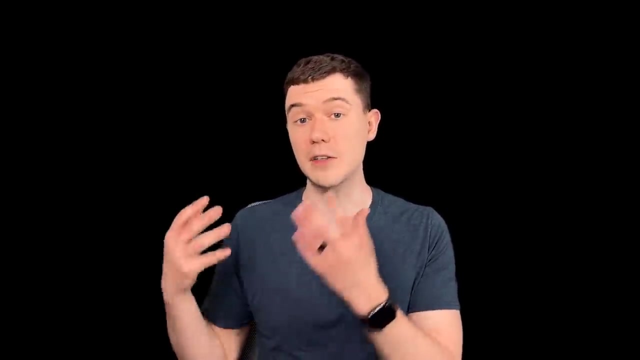 The birthday problem, or the birthday paradox, is a fascinating piece of mathematical probability theory that illustrates how bad humans are at estimating probability and statistics. Here's the question: How many people need to be in the same room such that the probability of two people having the 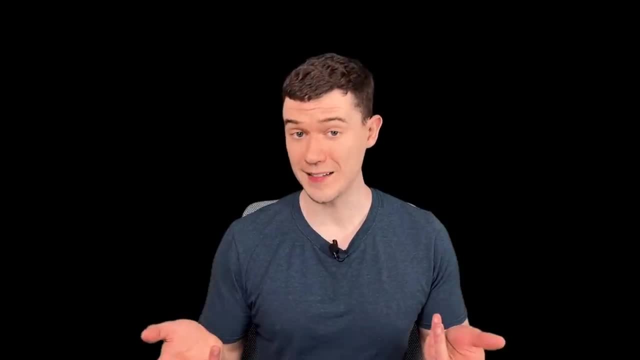 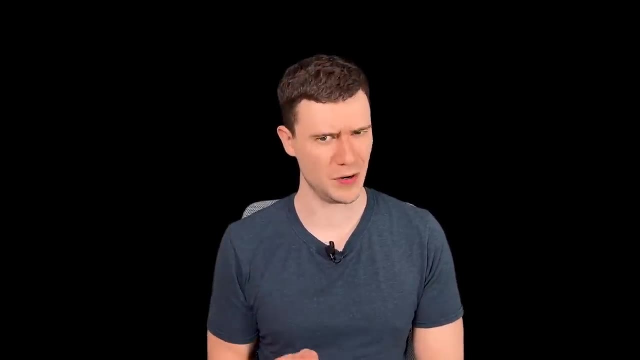 same birthday is above 50%. Wanna take a guess. Maybe you think 100, maybe a little bit more. The answer is 23.. That's right. it only takes 23 people in the same room to have a greater than 50% chance. 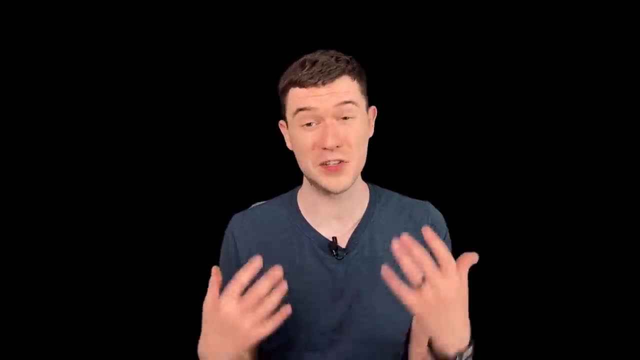 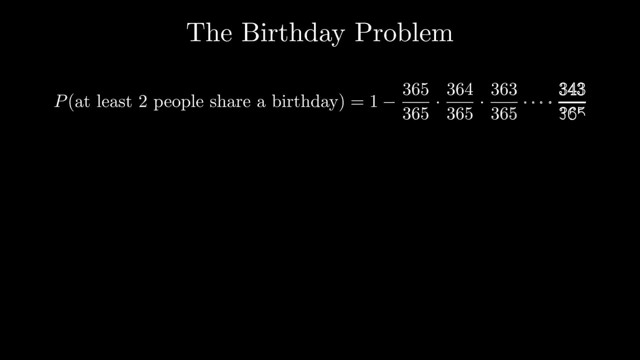 that any two people have the same birthday, which is extremely counterintuitive. But all you need to do is work out the combinatorics and the probability, and there it is. I think what most people confuse this with is the probability that you yourself. 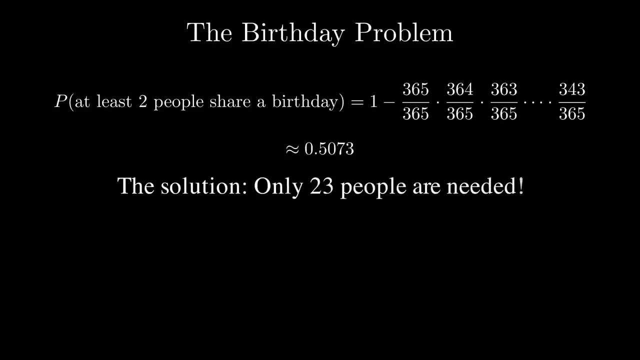 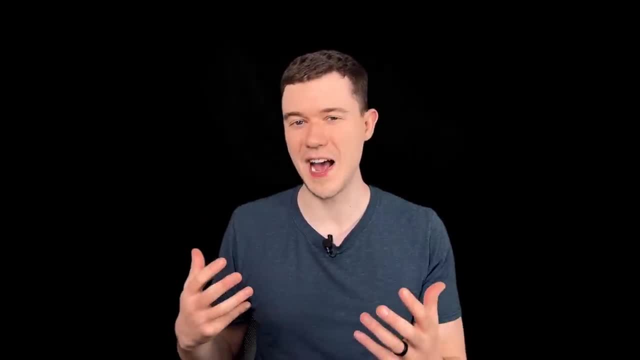 has the same birthday as someone else, That's much more unlikely. But the question's asking: do you share a birthday and does anybody else in the room share a birthday? And when you think of it like that, the odds get much higher. 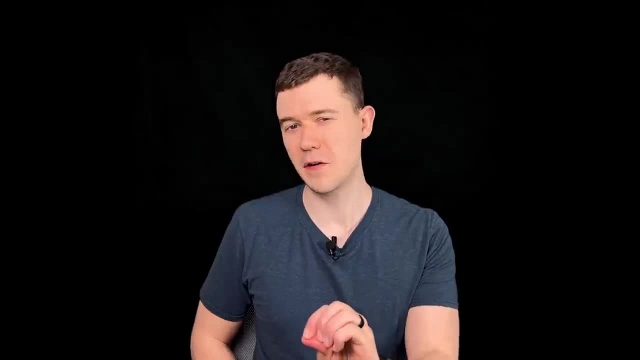 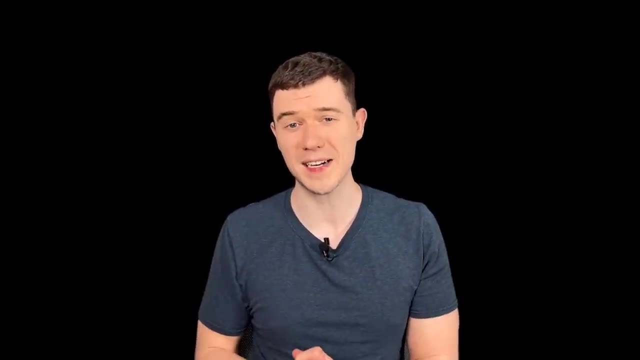 Time for some mispronunciation. The Banach-Tarski paradox says that if we take a solid sphere and decompose it into finite pieces, we can put the pieces back together in such a way that it creates two solid spheres of the same size. 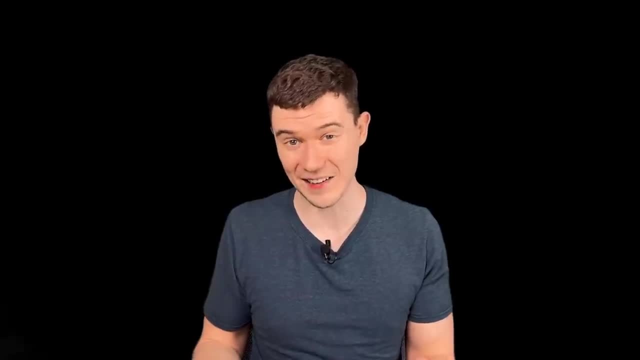 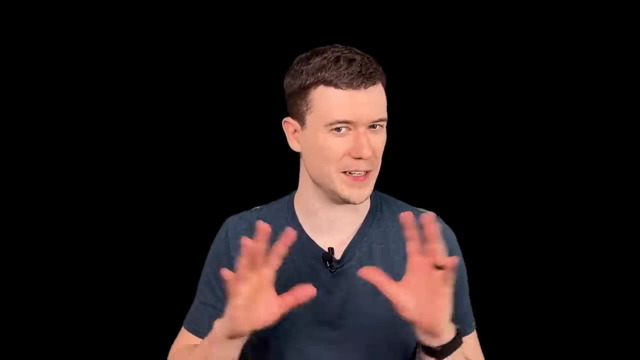 How can that be? Well, I'm not gonna get into the details, but set theory and the axiom of choice prove it to be so. When I was trying to make the animation for this, it did not turn out how I wanted it to at all.